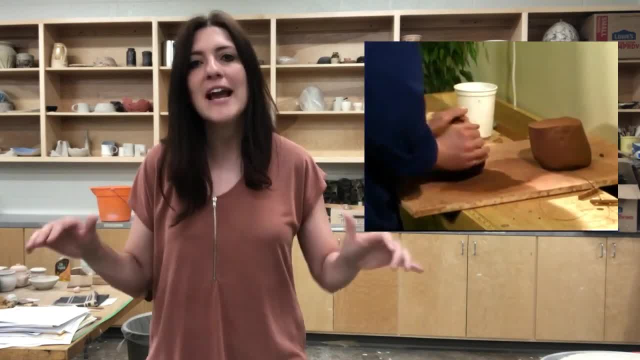 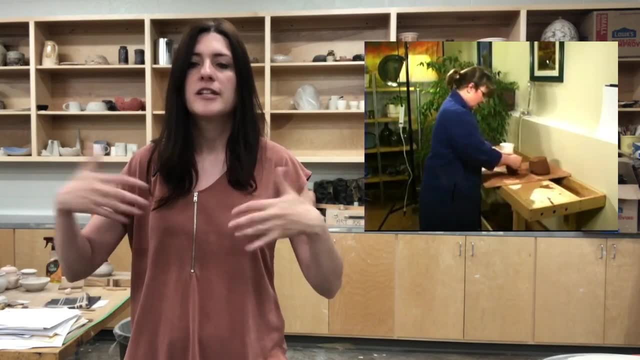 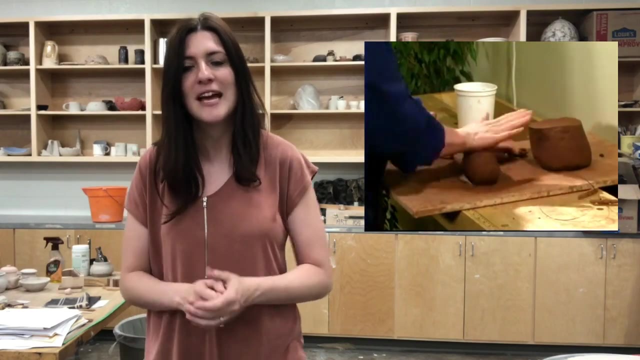 must do when working with clay is remove all the air pockets inside the clay. You may not even be able to see the air pockets, but if they're there, things might explode in the kiln later on. So it's important to just go ahead and remove these air pockets there in the first step. 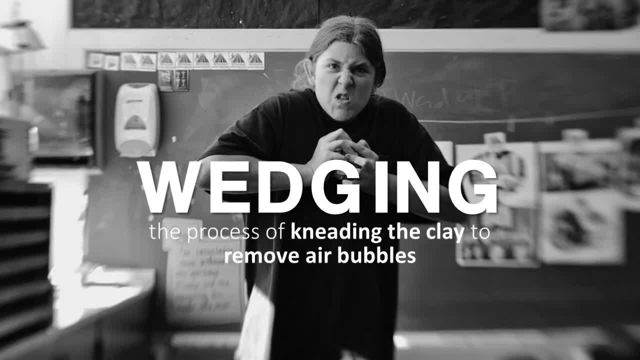 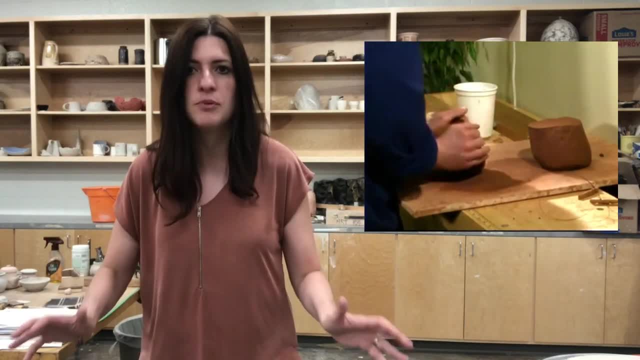 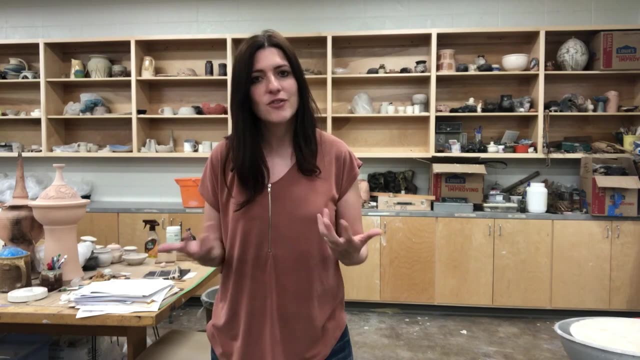 It's a process called wedging. Now, to wedge your clay, you can throw or knead the clay by pressing down on it and rolling out any possible air that may be inside. Now, once you do that, you can start working with your form. There are a few things to remember when working with clay. 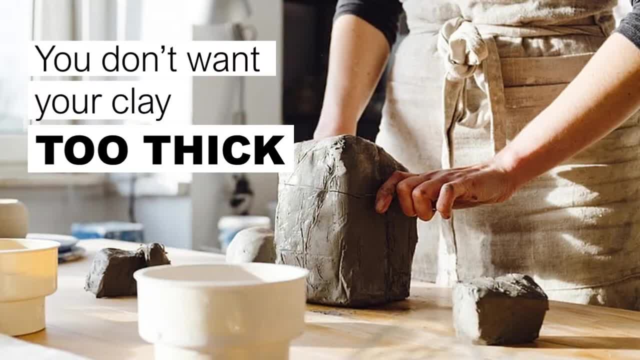 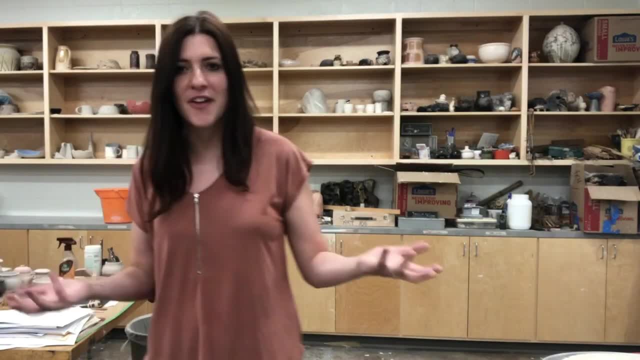 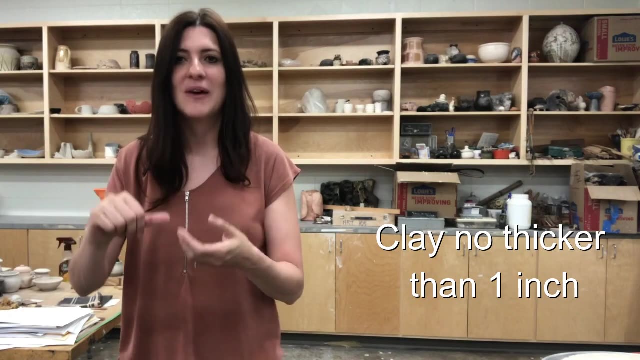 One. you don't want your clay to be too thick. The thicker it is, the more likely for air to be trapped inside. So a typical rule of thumb is that your clay should not be thicker than your thumb, or no more than one inch, okay. But at the same time, clay can be fragile and thin. 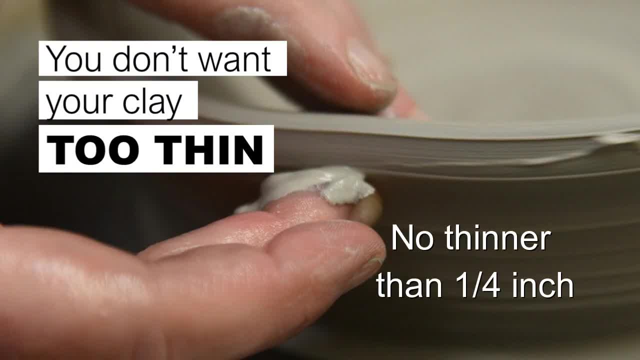 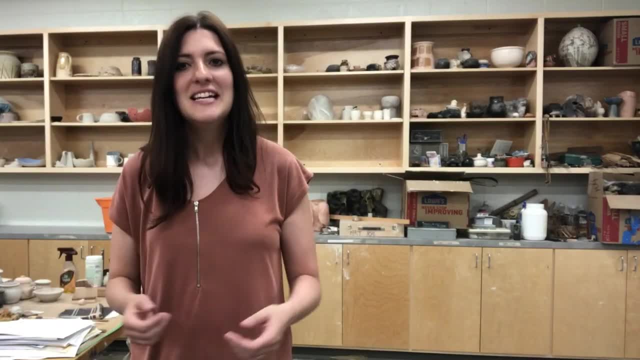 parts can break, So you also don't want your clay forms to be thinner than about a quarter of an inch. So those are important things to keep in mind As you're working with clay. if you need to attach two separate pieces, you actually need to make sure that you have the right amount of 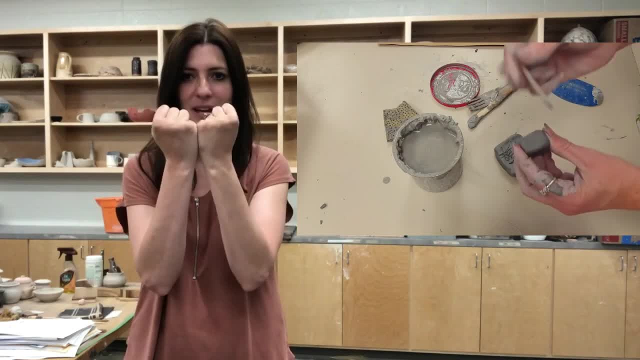 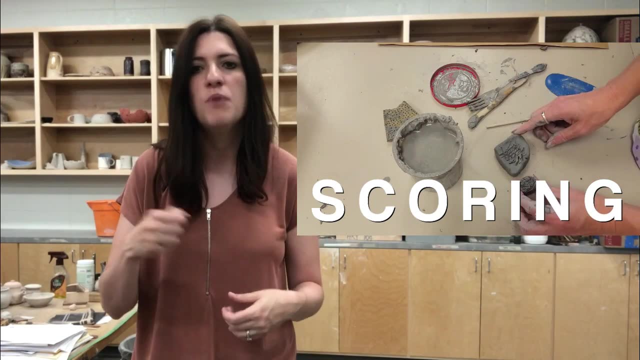 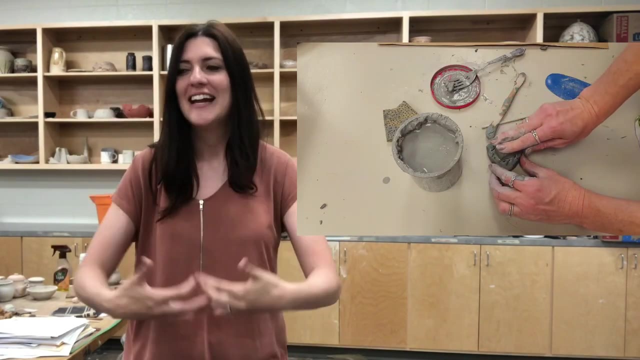 clay. You really have to create a rough surface at the attachment points of both of these pieces. This is called scoring, and you can score your clay by scratching into both sides, adding a bit of water and then attaching the pieces. This will kind of help interlock the forms together. 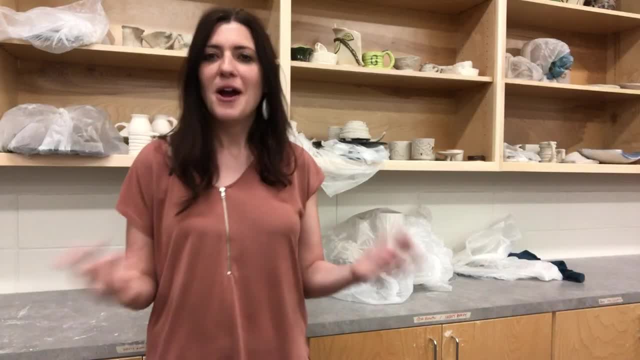 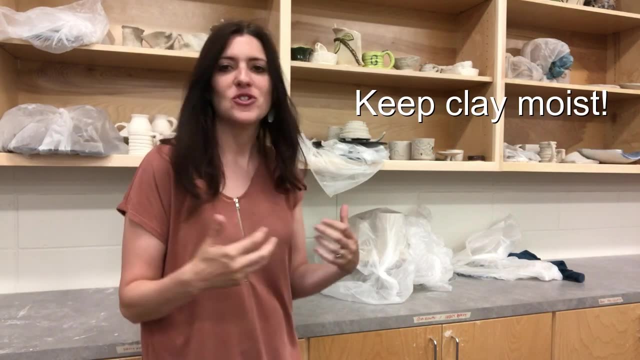 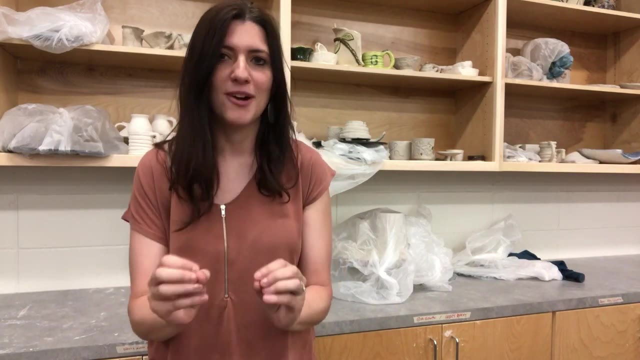 and will prevent detachment later on. Throughout the process. it's important that you keep your clay moist. You don't want it to dry out and then be forced to start all over Now if you want to work on your project over multiple sessions, you can prevent your project. 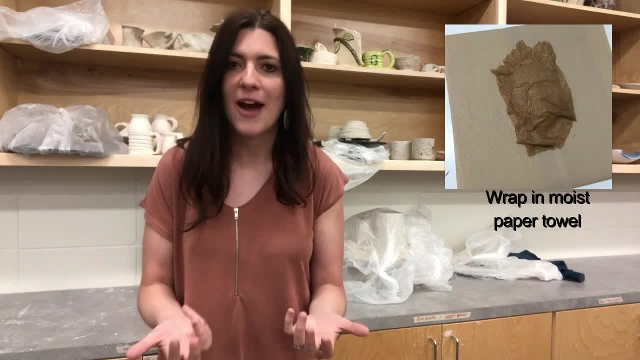 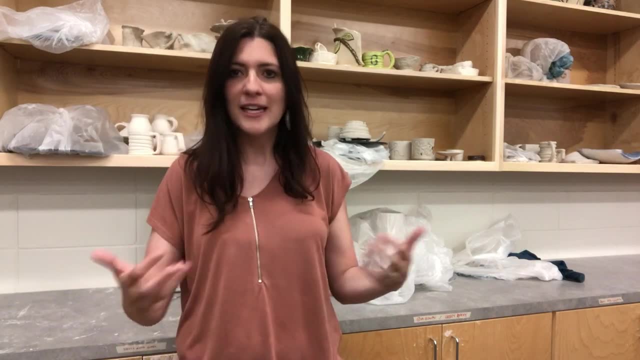 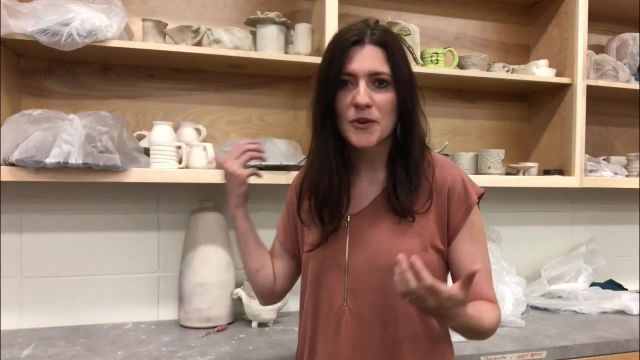 from drying out by wrapping it in a moist paper towel and then covering it in a plastic bag. This will help keep the air out and, hopefully, keep your clay moist, allowing you to pick back up where you left off. When an artist is completed with their project, they will need to let it dry. 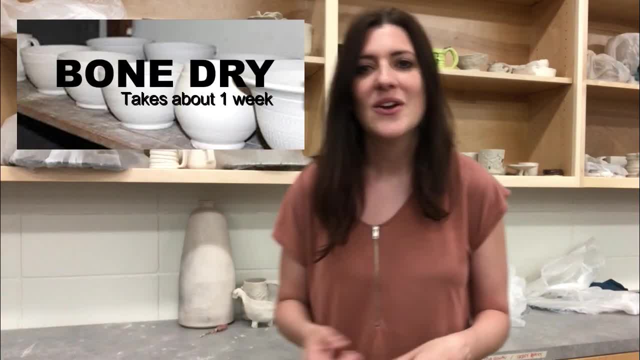 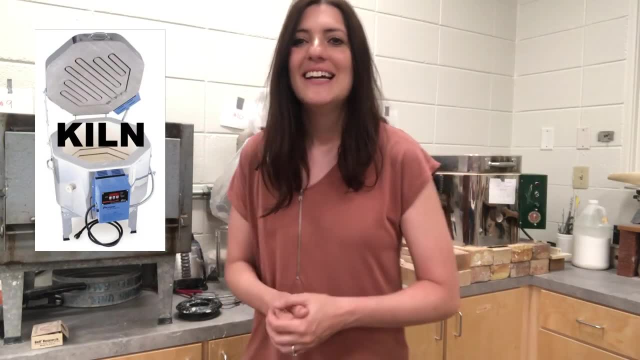 out until it reaches bone dry status, which can take about a week or so. So if you're working with clay for a week and then when the clay is dry, it can be put into a kiln. A kiln is a special kind.